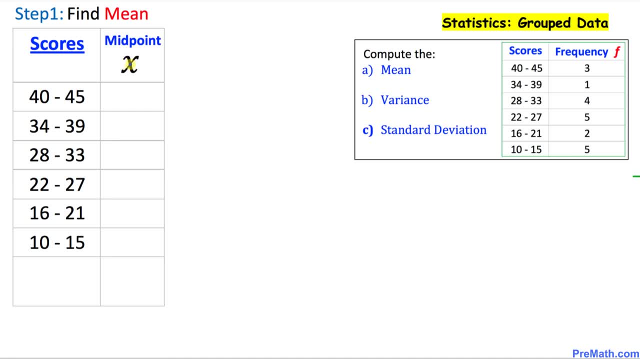 going to calculate the midpoint, which is called an x, between these points between 40 and 45. let me show you how to do this one. to find the midpoint of these 40 and 45, just write them down: 40 plus 45, and always divided by 2, that is going to give us 85 divided by 2 equals to 42.5. let's write it. 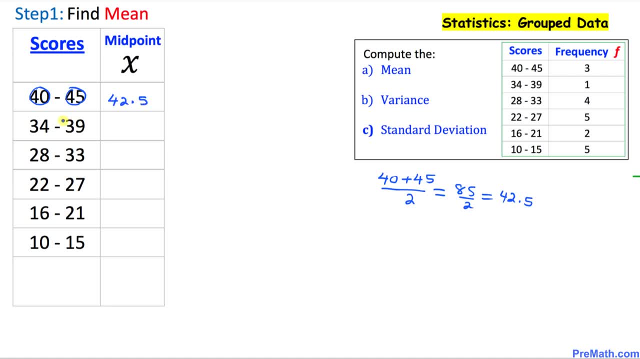 down 42.5. to get the midpoint between these two points, let's add them up and divide by 2 and we are going to get 36.5. and if we find the midpoint between these two points, add them up and divide by two. that is going to be 30.5. 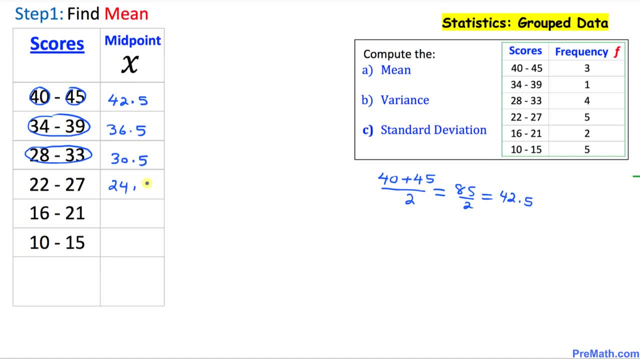 likewise, that's going to be 24.5,, 18.5 and 12.5. and here are the frequencies that i've just copied down from our original equation. from here and now, in the next table you will be able to identify, four have been given an two to get the word holgang. 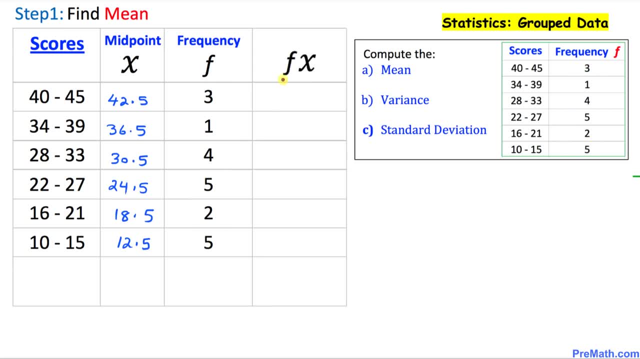 four. those that you get is going to be decimal. current period. 魔并 lag column. we are going to multiply the frequency F with midpoint X. let's go ahead and multiply. frequency is three times forty two point five. if we multiply these two, we are going to get 127.5, and if we multiply one time. 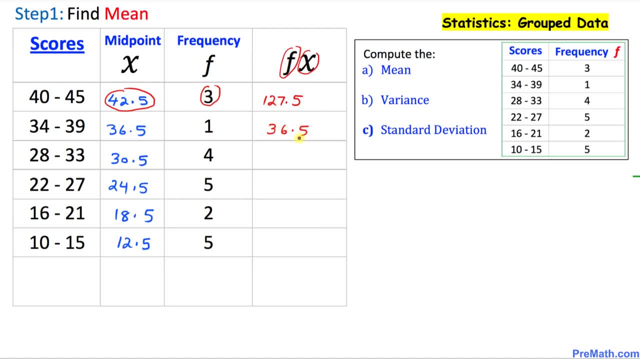 thirty six point five. that's going to give us thirty six point five, and the next one is going to give us one hundred and twenty two. this is going to be one twenty two point five, this is going to be thirty seven, and here it is going to. 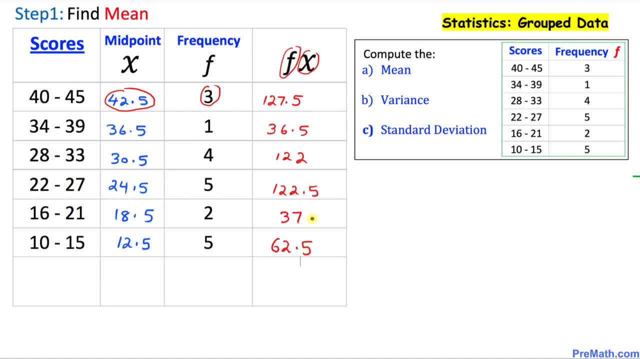 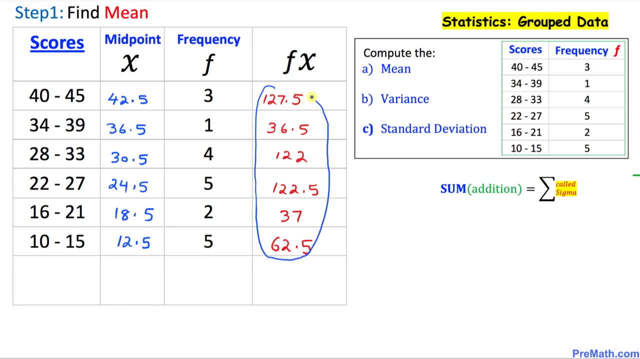 be sixty two point five. and now we are going to add up all these values in this fourth column. if we add them up, I am going to use Sigma rotation. Sigma of F of X equals to: if I add these values, that is going to give us five zero eight. once again, this. 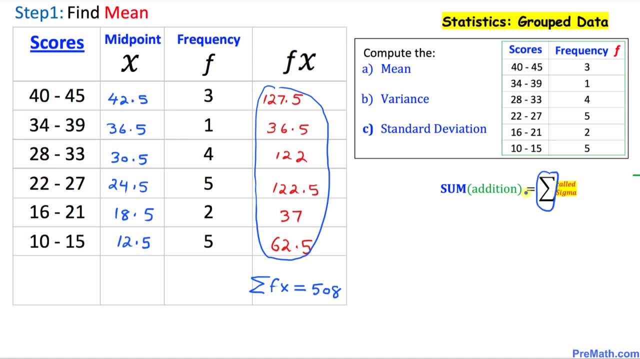 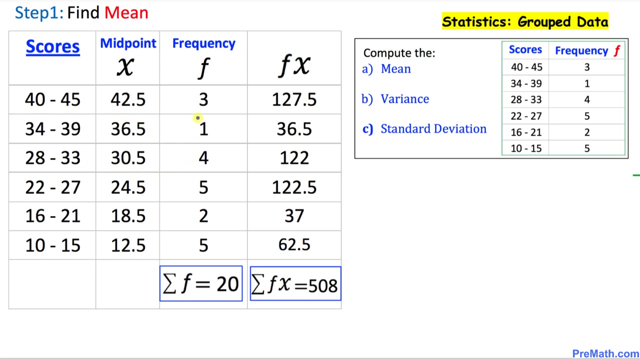 notation is called Sigma, which really means some or sometime. we call it addition. and one more thing: if we look at these frequencies column, we are going to add these value up as well, so we can use: Sigma of F equals to simply 20, and here is our final product. i have nicely filled out. 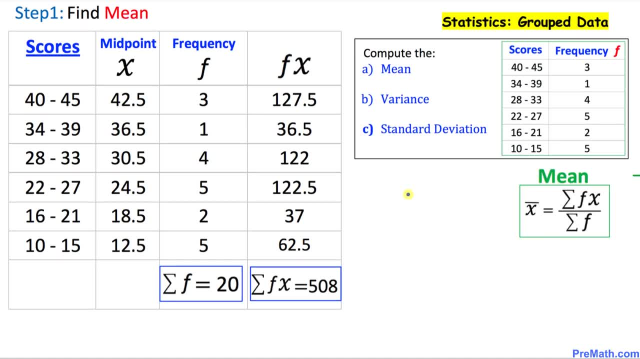 these value in this table. and now, finally, you, we can calculate the mean that is represented by X bar. so X bar equals to this formula. so this: on the numerator Sigma of F of X, we already calculated that one that is five zero eight divided by Sigma of F in our 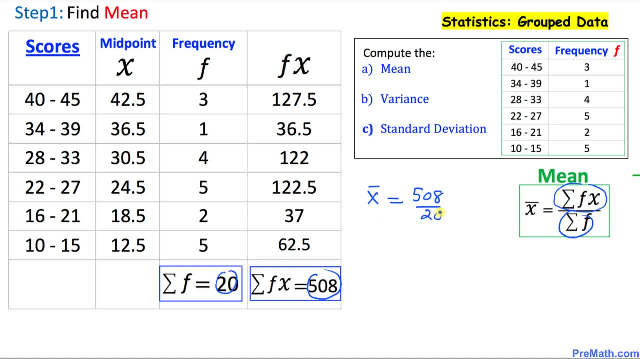 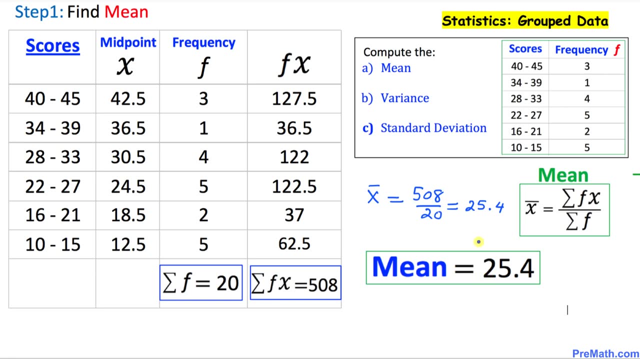 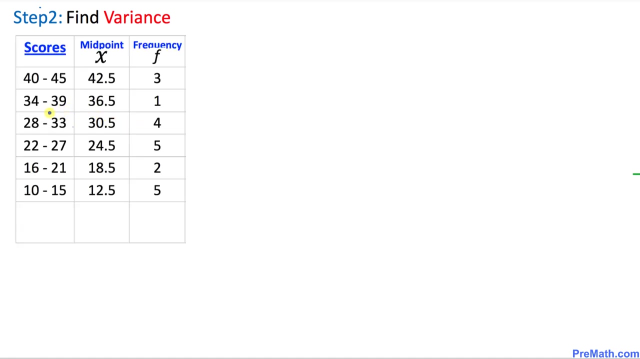 case is 20, and if we divide this one, that is going to give us twenty five point four. thus, our mean turns out to be twenty five point four. and now, in our step to, we are going to calculate the variance, and from our previous steps, we know the. 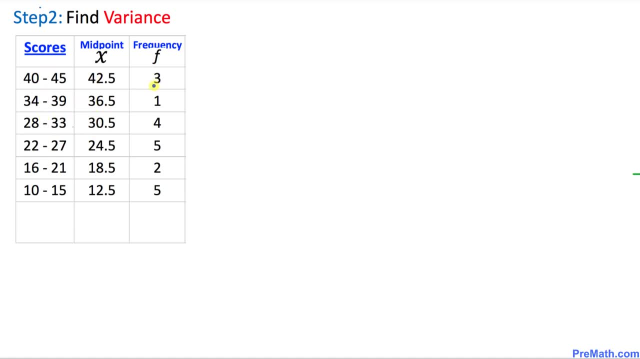 score values, the midpoint x and the frequencies. as you can see over here and in our next column, this is for mean x bar. we're gonna fill it in and from the step we figured out, the mean equals to 25.4. let me just write it down over here. 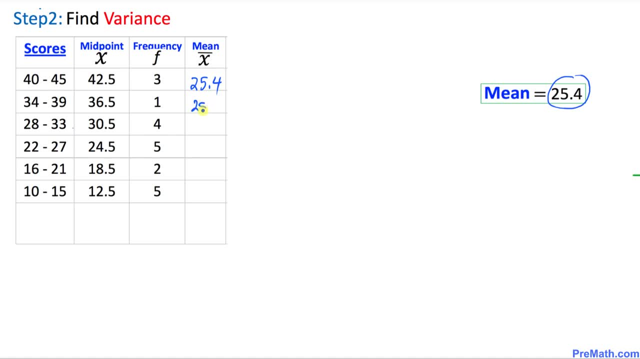 25.4 across the board: 25.4, 25.4, 25.4. and now, in the next column, we are going to find the difference between x and x bar, x minus x bar. let's go ahead and do this one: this is our x value and this is our x bar. we're going to subtract this one. it is going to give. 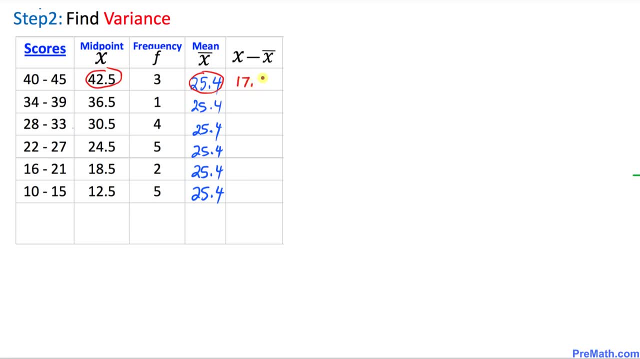 us, if we subtract 17.1, and if we subtract this minus this value, that is going to give us 11.1 likewise. so we're going to get 5.1. negative 0.9, negative 6.9 and finally negative 12.9. 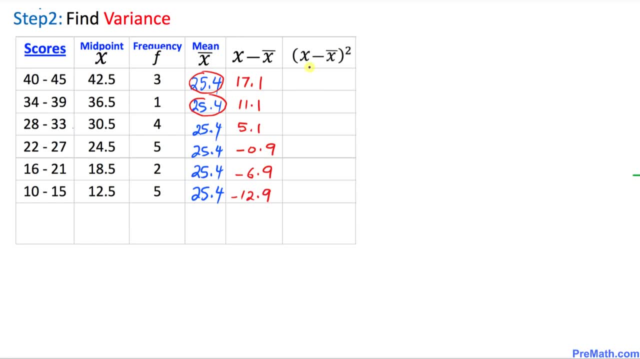 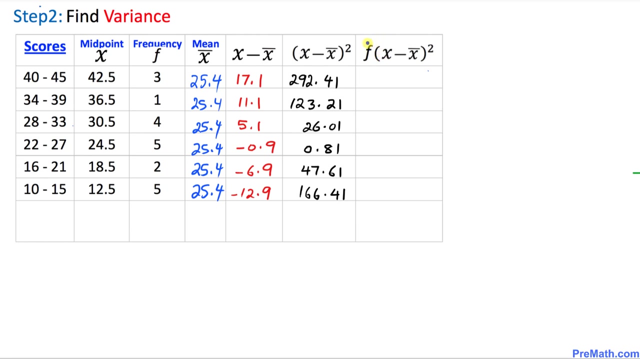 and finally, in this next column, we are going to square these values that we figured out in our previous column. if we square these one, we are going to get 292.41, 123.21, 26.01, 0.81, 47.61 and finally 166.41. and now, in the next column, we are going to multiply the frequency. 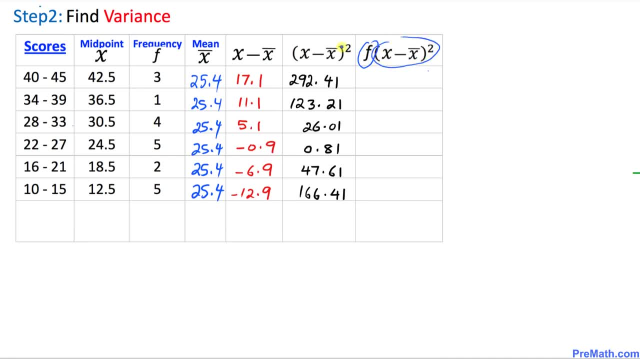 f times x minus x bar square. that means we're going to be multiplying these columns, this frequency column and this square column. okay, let's multiply these numbers three times 292.41, we are going to get- we have to be very careful with these calculations now- 877.23. likewise, if we multiply the next numbers, we're going to get 123.21, 104.04. 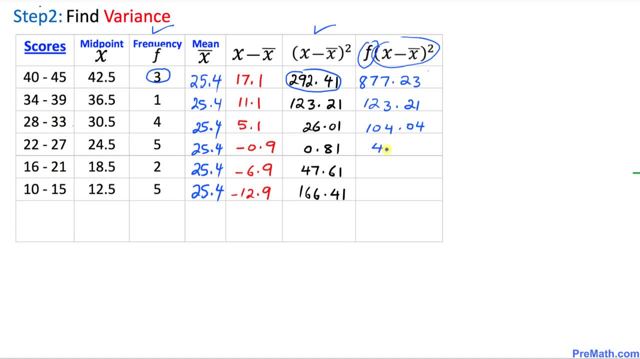 the next one is going to be 192.41, and then we're going to get 192.41, and then we're going to get 4.05, and next one is going to be 95.22 and finally that is going to be 832.05. 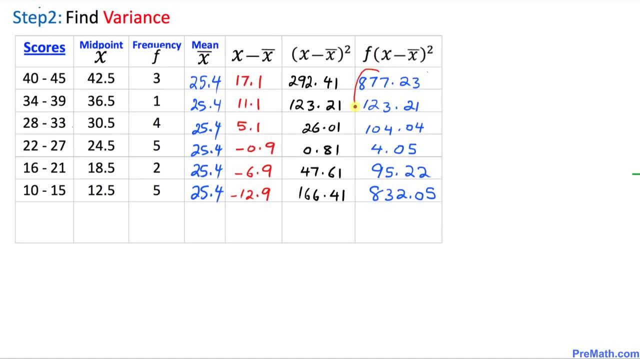 and now, in the next step, we are going to add up all these values in this column, and so when we add them, we're gonna use the sigma notation over here. this is going to be f times x minus x. bar square equals to: that is going to be 2035.8. and likewise we're going to be: 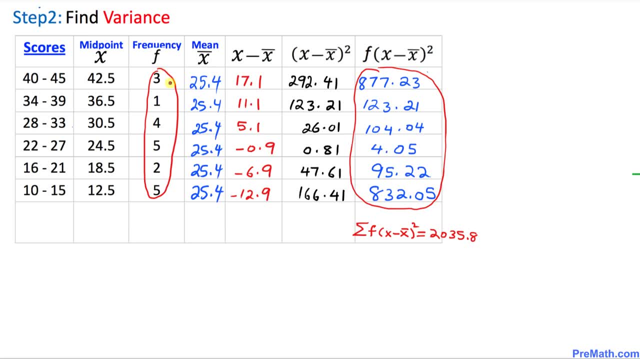 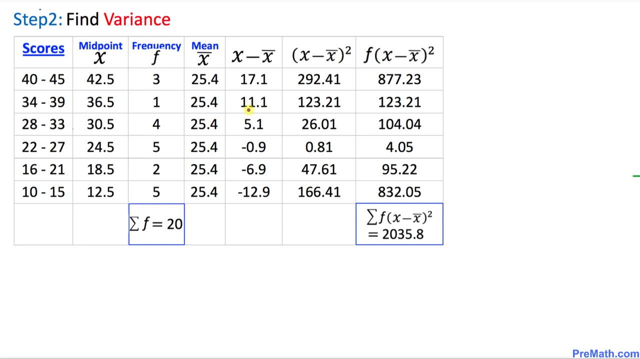 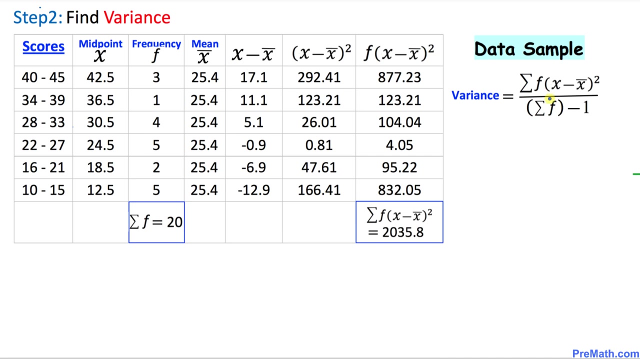 adding these frequency values as well. so we're gonna say Sigma of F equals to 20, and here is our final product. I have just put down these number in a nicer way, and now we'll be able to calculate the variance by using this formula. and one thing: just keep in your mind that we 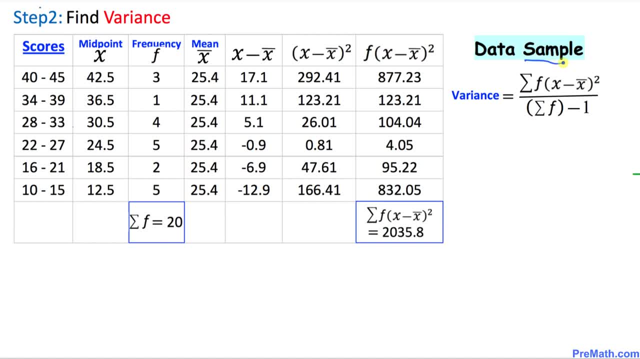 will be using this data as a sample. okay, just keep in your mind. so the variance- let's go ahead and calculate variance- equals to: on the numerator, this thing you can see is same as this quantity. let's put it down. so that is 2035.8 divided by. 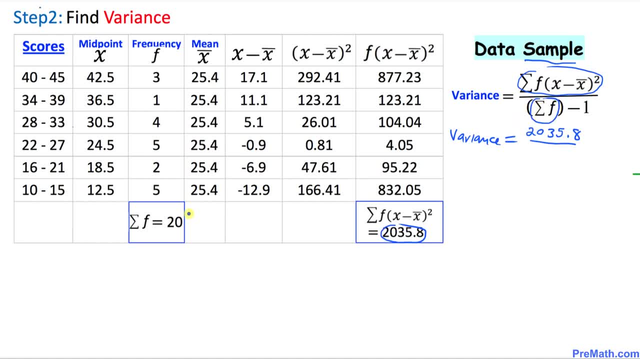 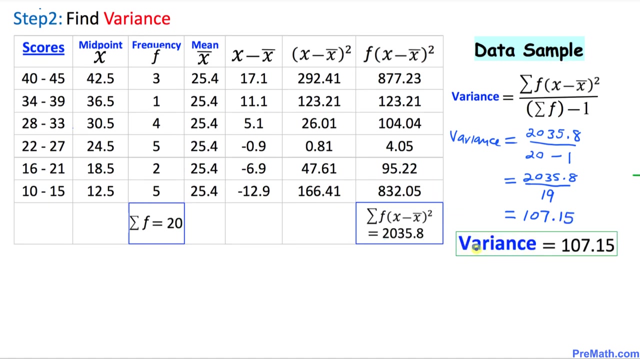 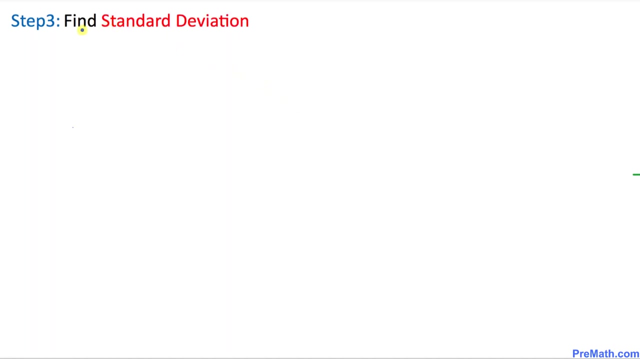 we have a sigma of f in our case- is 20. you write down 20 and then minus 1. let's simplify this one: 2035.8 divided by 19, and that is going to give us 107.15. so that's our variance turns out to be 107.15. and finally, in our step 3, we are going to calculate. 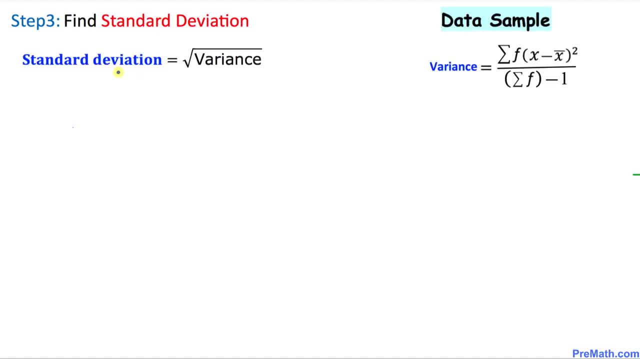 the standard deviation, and here is the formula that we'll be using. standard deviation is always equal to the square root of the variance, and here is the variance formula over here. and this, once again, is the sample data set. and here's the variance value that we figured out in our previous step.